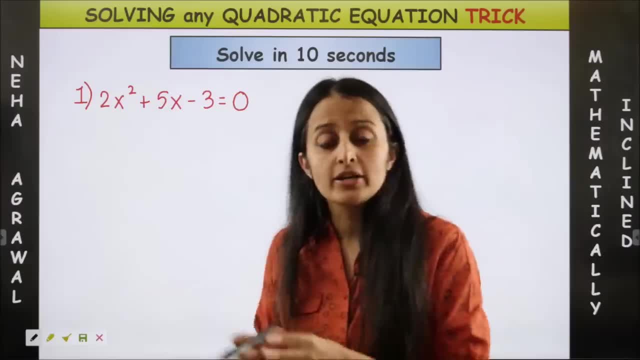 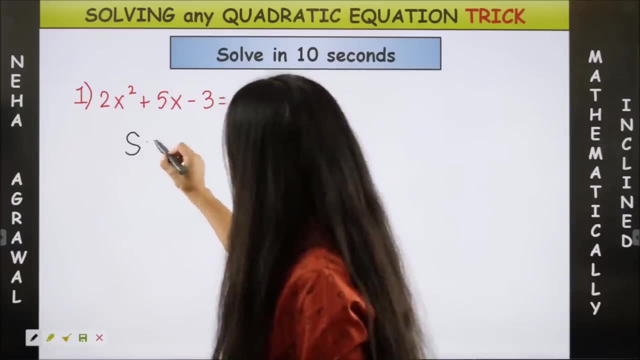 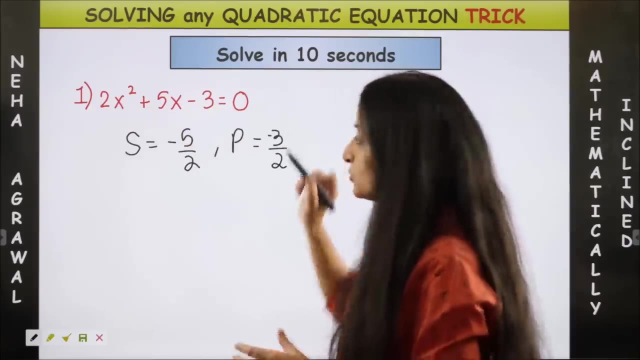 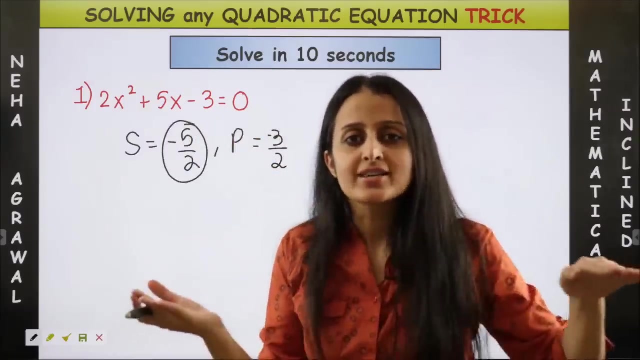 basically factorizing any quadratic equation is when you talk of sum of its roots and product of its roots, Right. the sum of its roots is –bh, as we can see, and product is ch. that gives us –3. Now, Now all you need to do is take the sum. yes, take the sum and just take its half, absolutely. 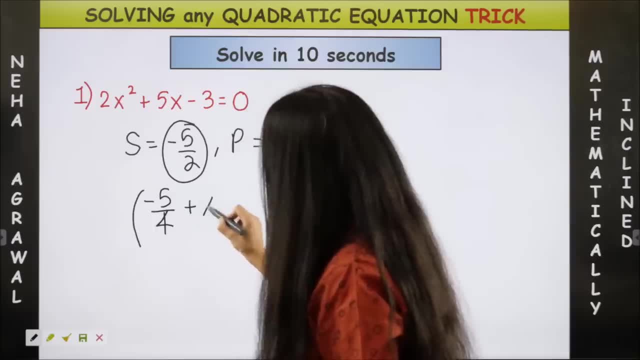 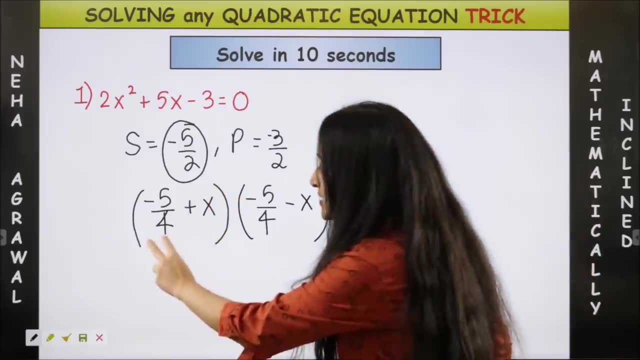 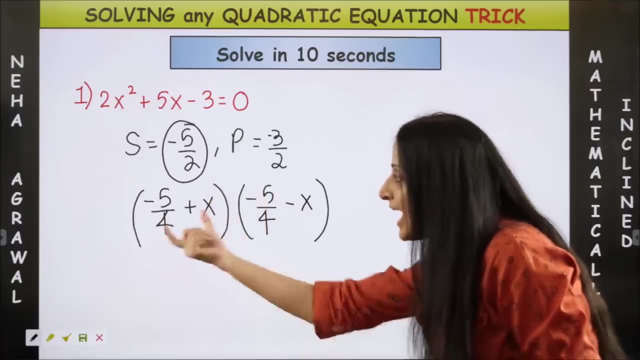 so minus 5 by 4. just add the factors plus x and minus x. so now my factors have become minus 5 by 4 x, minus 5 by 4 plus x and minus 5 by 4 minus x. why? because when you add them, 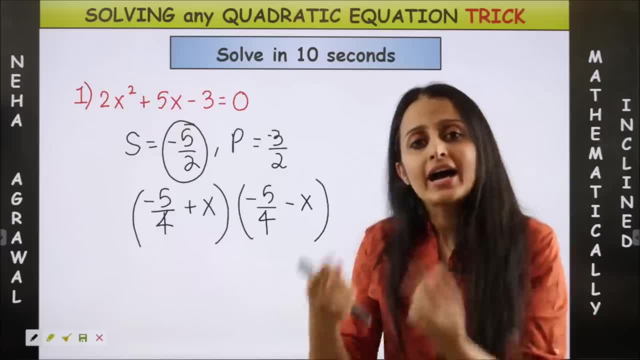 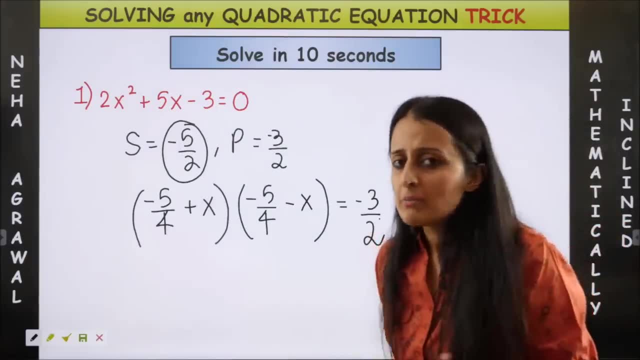 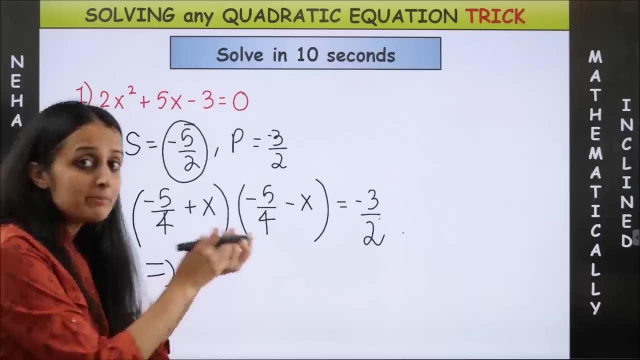 up, you will get minus 5 by 2 and the idea is, when you take their product, it should give you this. that's all what we need to solve now. you will think this is another quadratic, but, guys, if you watch it closely, it is just the format a plus b, a minus b. so this simply. 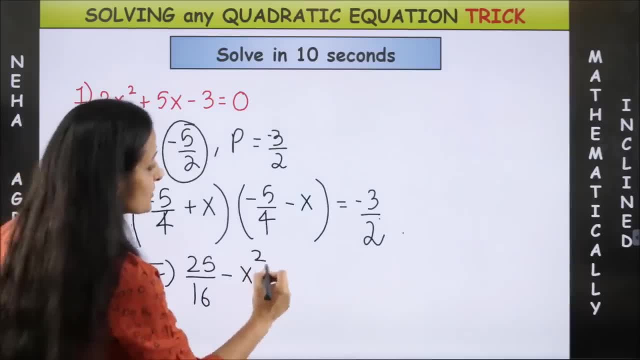 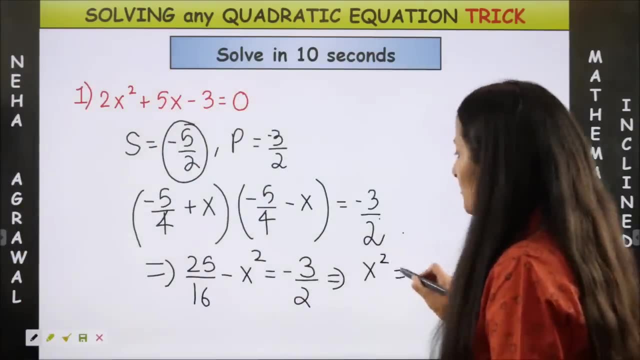 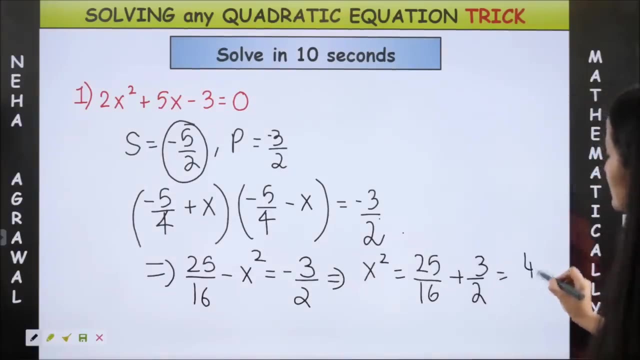 becomes a square minus b square right. so when you will solve this one, your x square base becomes, you can say 25 by 16 plus 3 by 2, which on solving gives us 49 by 16. yaani ke, your x is simply plus minus 7 by 4. now take any of them, whether 7 by 4 in both the factors. 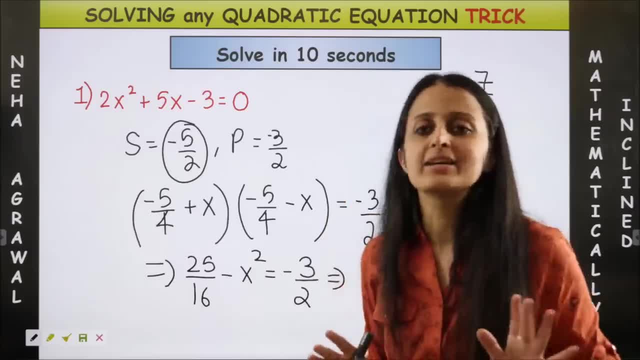 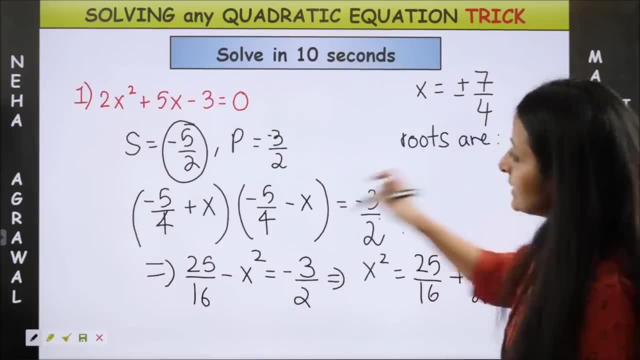 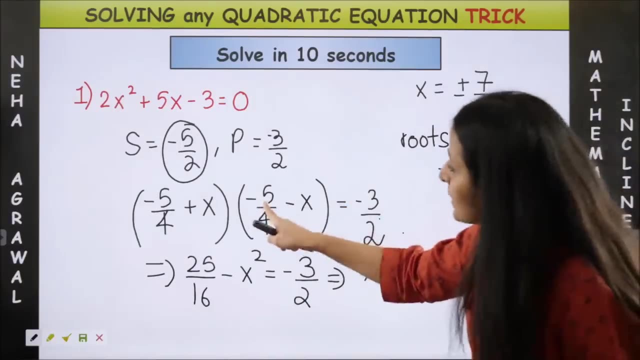 or minus 7 by 4. trust me, you will end up getting the same answer if I take x as 7 by 4. so my roots are 7 by 4 minus 5 by 4 plus 7 by 4. that makes it 2 by 4, so half. and minus 5 by 4 minus 7 minus. 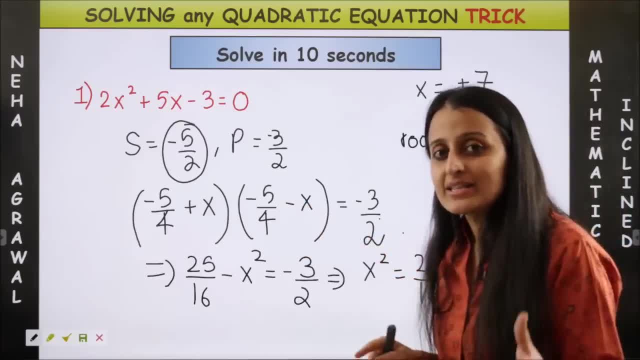 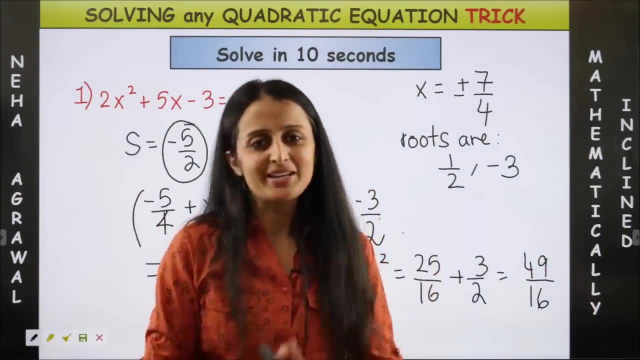 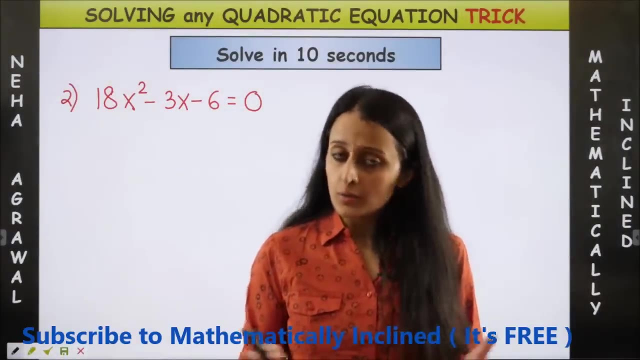 5 by 4 minus 7 by 4, that makes it minus 12 by 4 minus 3. bingo, these are the roots of the quadratic equation. please make a note. now. you might feel, boss, we can anyway factorize using middle term splitting. well, you can of course go ahead and do that, but you can of. 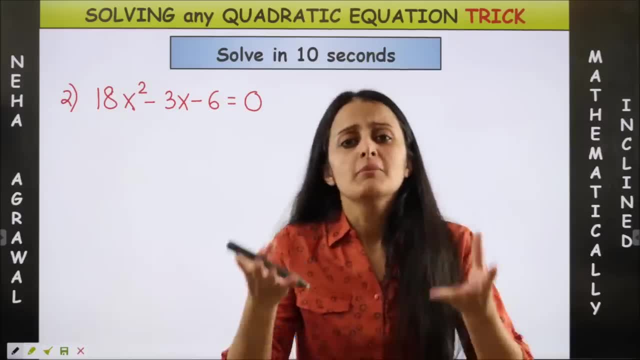 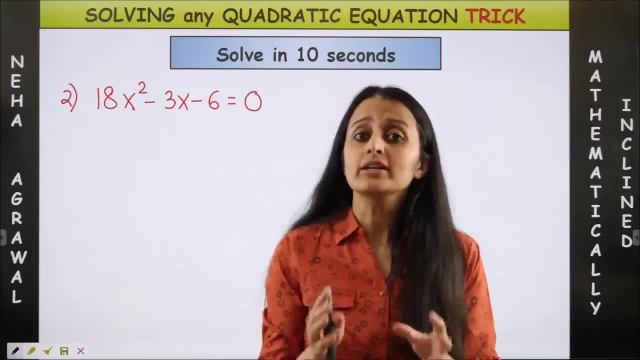 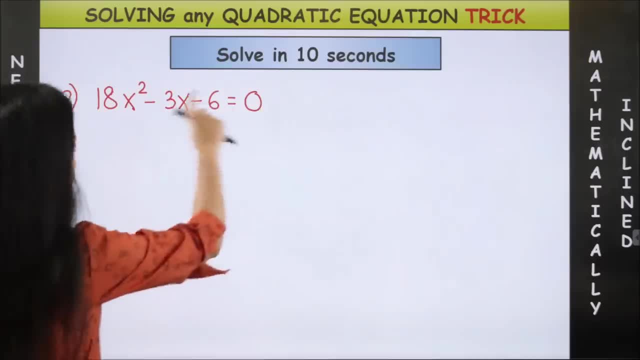 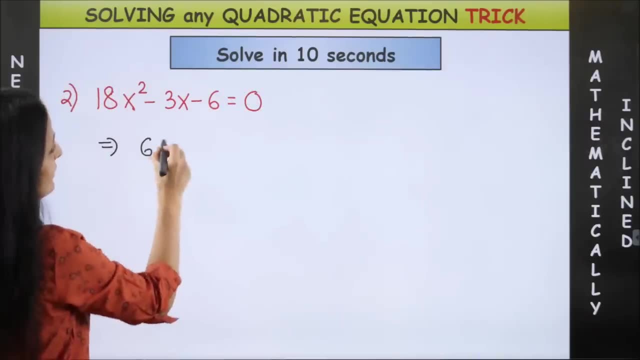 get to the roots super quick. so watch this out now. first of all, you know, let's just simplify this one right. so you know if you take six, you know if you take three, common, this anyway just becomes this now: sum, sum is again minus of this one. so one by six product is minus. 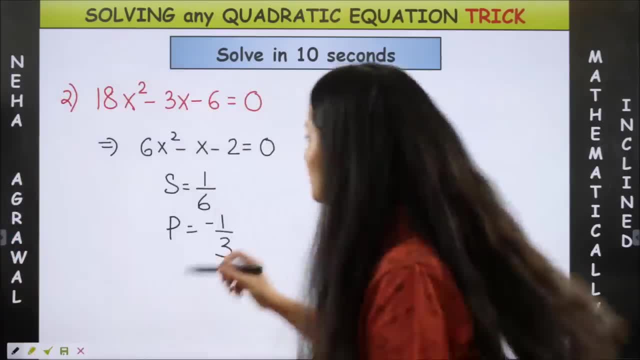 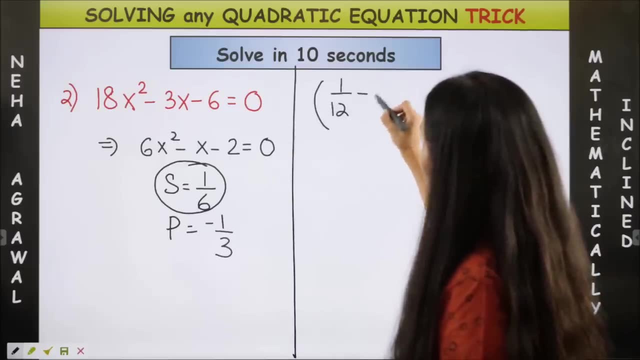 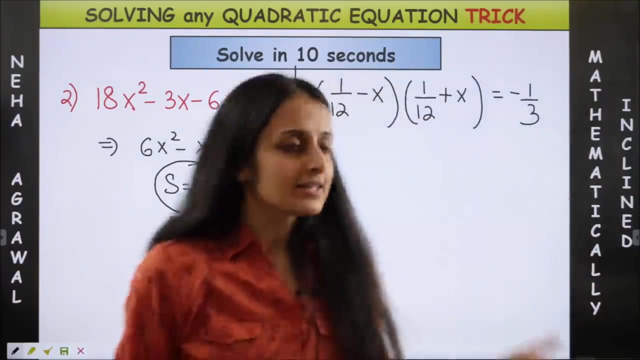 2 by 6, so minus 1 by 3.. All you need to do is take its half. Yes, just take its half, so that will be 1 by 12 minus x, and 1 by 12 plus x is equal to minus 1 by 3.. That's it Now it is 1. 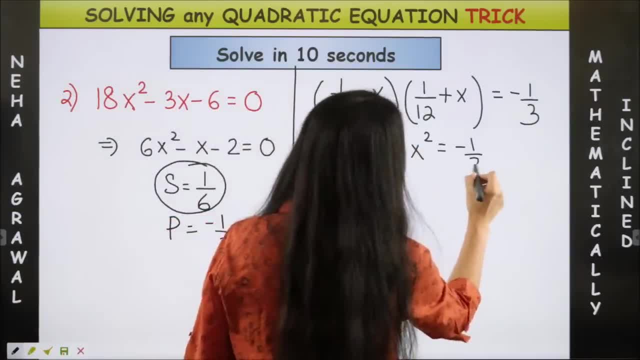 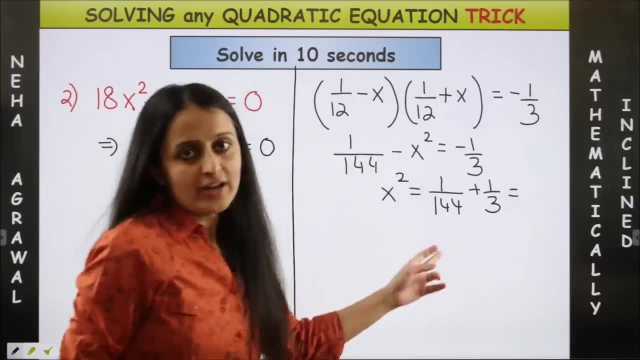 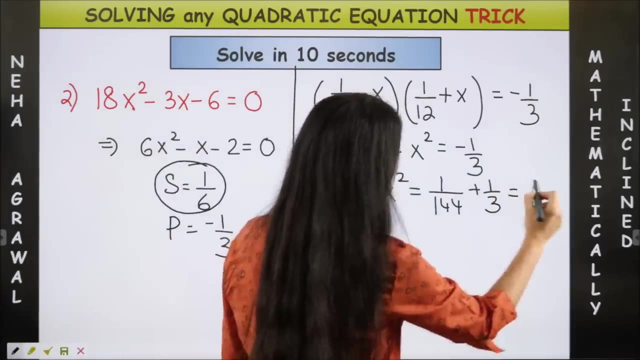 upon 144 minus x, square is minus 1 by 3.. So x square is, since 144 is a multiple of 3, so you know it's very easy now. This is going to give 48 plus 1.. So 49 by 144.. That means x is plus minus. 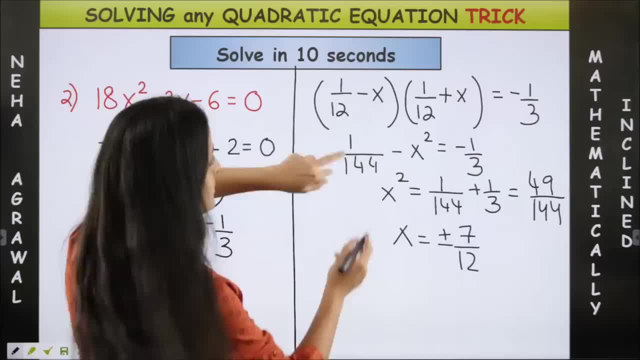 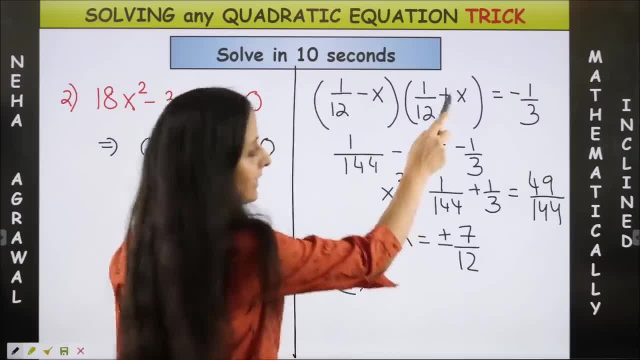 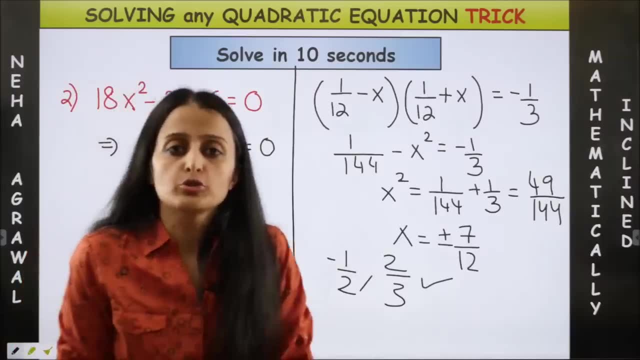 minus half. Again, it's minus half, And if you put 7 by 12 here, that gives us 8 by 12, which is 2 by 3.. Bingo, You've got your solutions. Please make a note. Okay, now this is getting really. 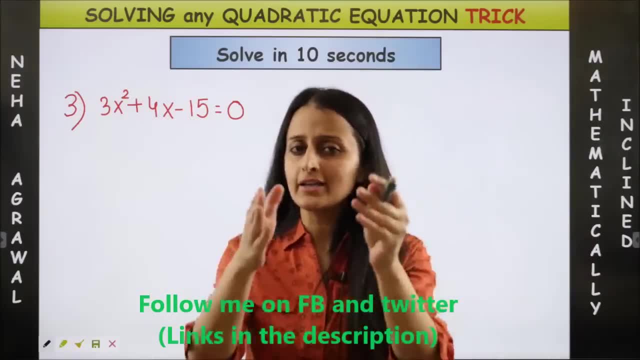 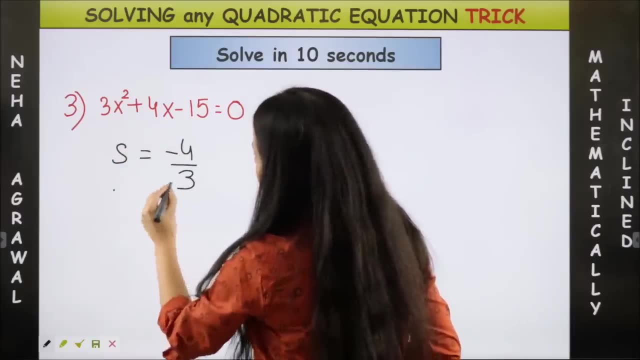 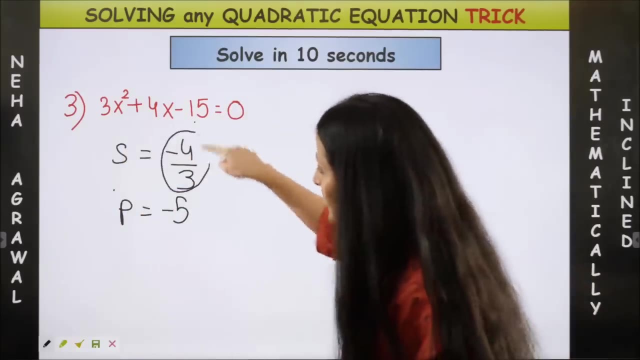 interesting. Now, this is a game of children and in fact a game of left hand. So you already know: the sum is minus 4 by 3.. Right, And the product will be minus 15 by 3. Which is minus 5.. All you need to do is take its half Correct, So that will make it minus 4 by 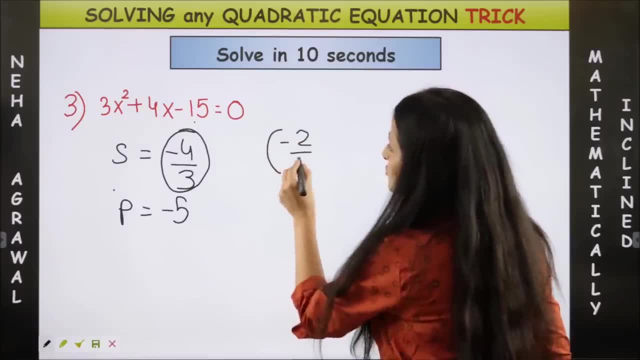 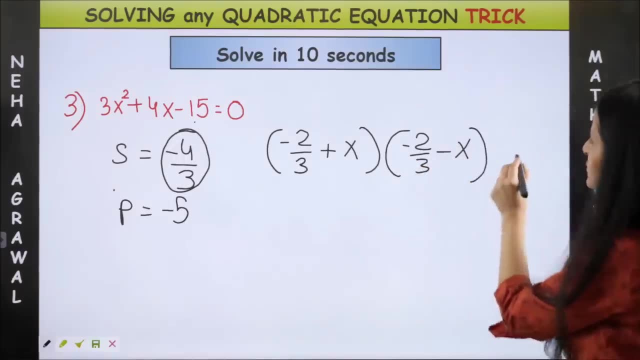 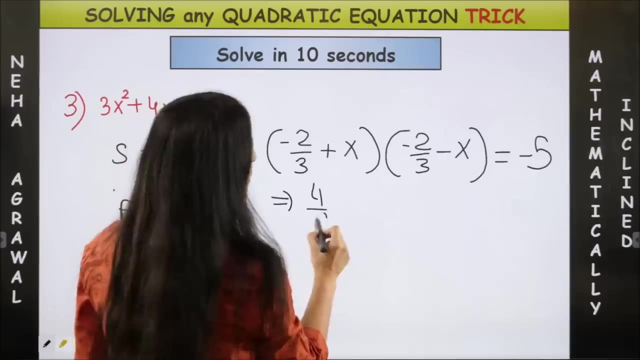 6. I mean minus 2 by 3.. So minus 2 by 3 plus x and minus 2 by 3 minus x is going to give me what Minus 5.. Now the same story, boss. This is going to give me 4 by 9 minus x square is minus 5.. I mean x square is. 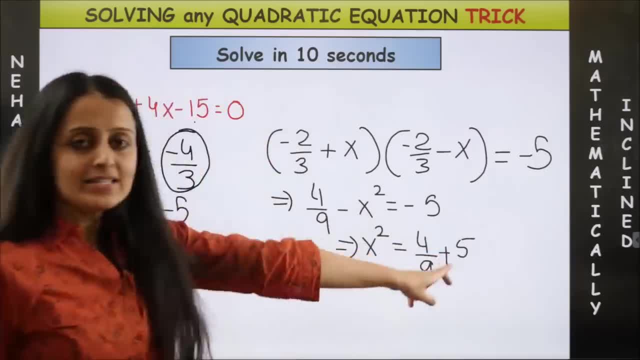 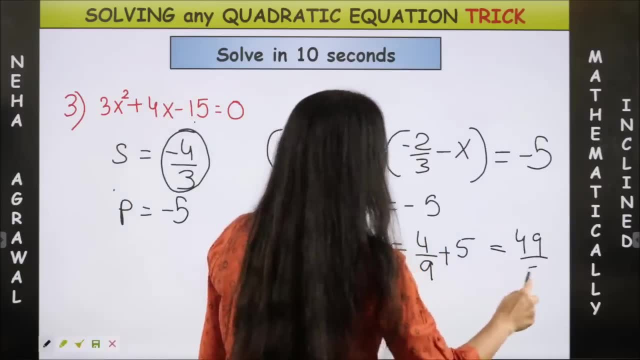 4 by 9 and x square is minus 5.. So this is going to give me 1 minus 2 by 12 plus x. Now this is by 9 plus 5.. As you take the LCM, this is of course going to be 45. So 49 by 9, that means 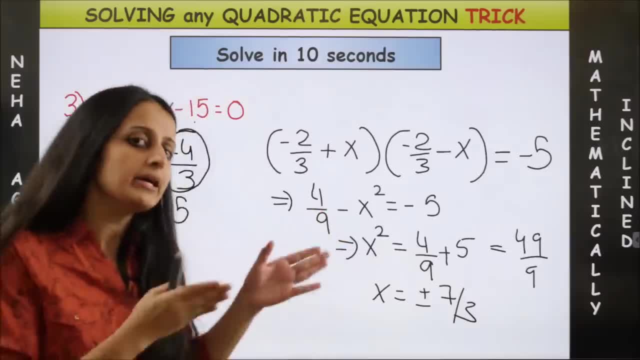 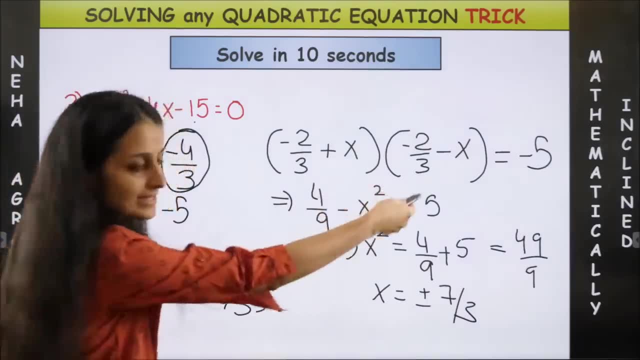 x is plus minus 7 by 3.. Repeat the same thing. What is your answer? It is simply 5 by 3 and minus 9.. This is minus 2 by 3, minus 7 by 3, which is minus 9 by 3.. 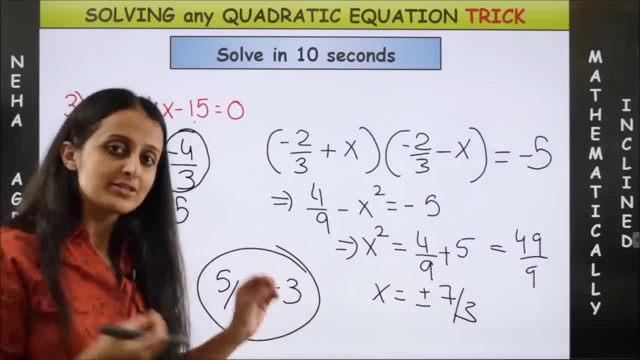 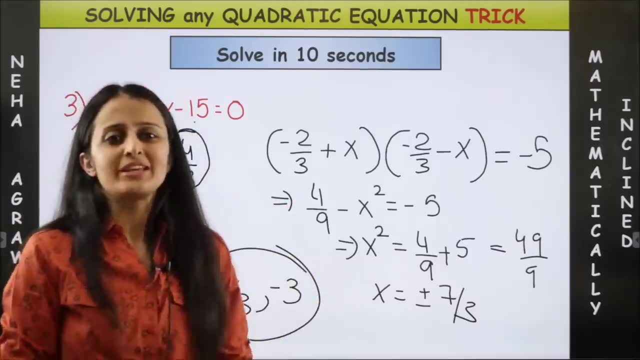 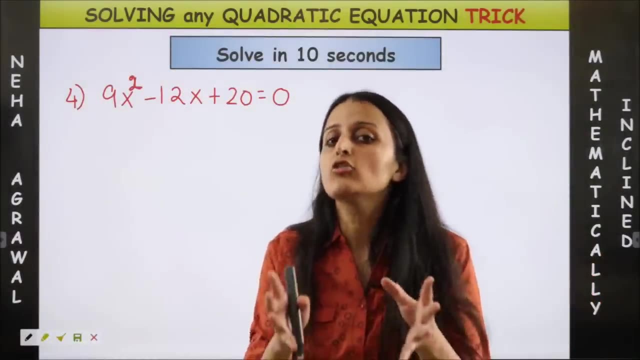 I am done. This is also sorted. I didn't even have to take 5 seconds to think about how to factorize, because it is so mechanical. Please make a note: All this has been perfect, ma'am, but what if you end up getting complex roots? How will you solve it so quickly? Well, 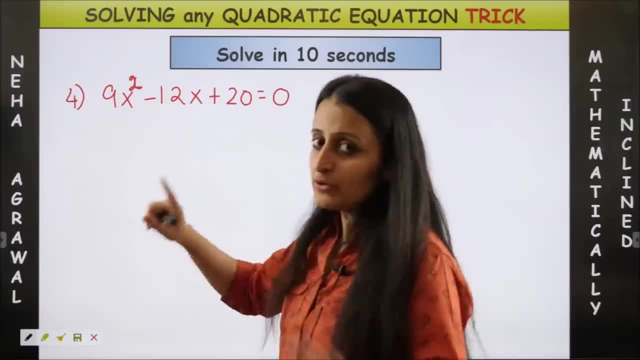 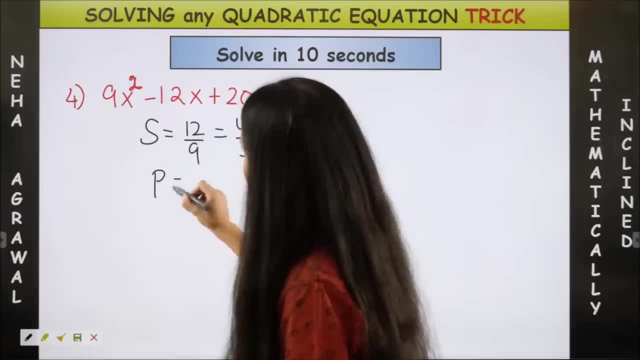 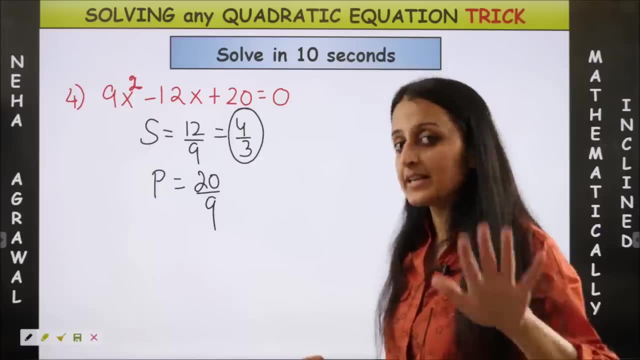 3. Yes, which makes it 4 by 3 and product will be 20 by 9.. Now the same story: when you divide it, it becomes 4 by 6, ie 2 by 3.. So this is going to be 2 by 3 minus x. 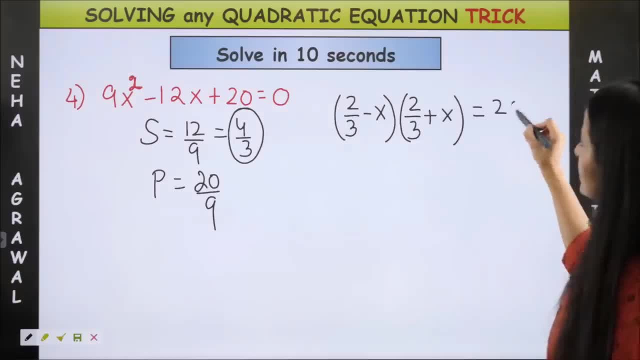 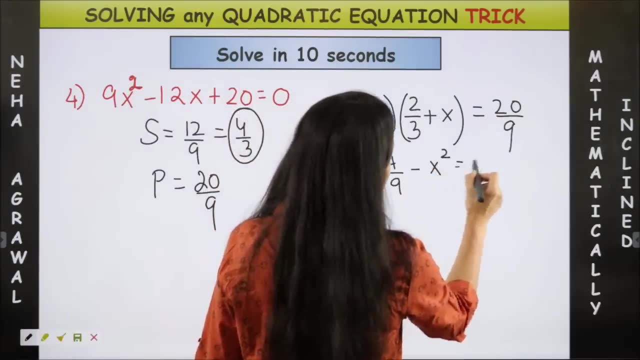 into 2 by 3 plus x is equal to 20 by 9.. Okay, Just keep solving with me. This is going to become 4 by 9 minus x. square is equal to 20 by 9.. ie, x square is going to be 4 by 9. 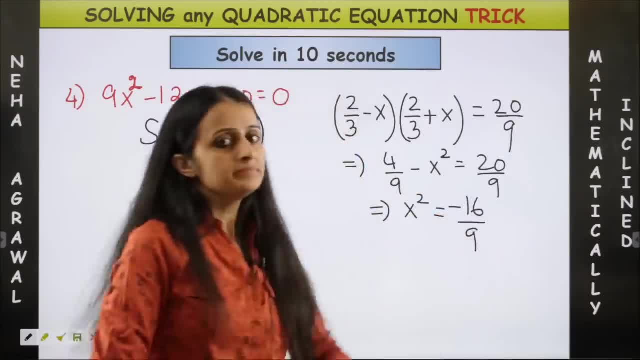 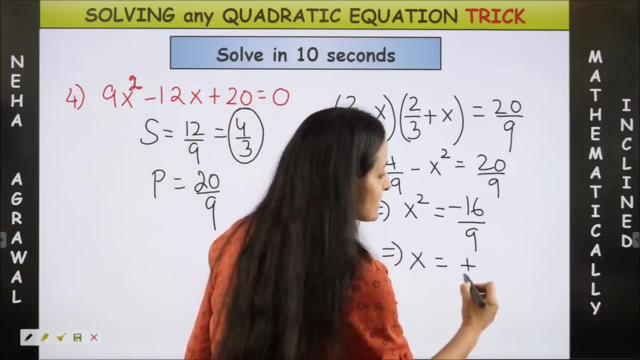 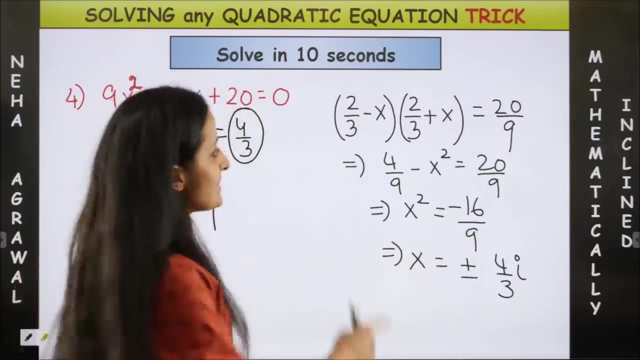 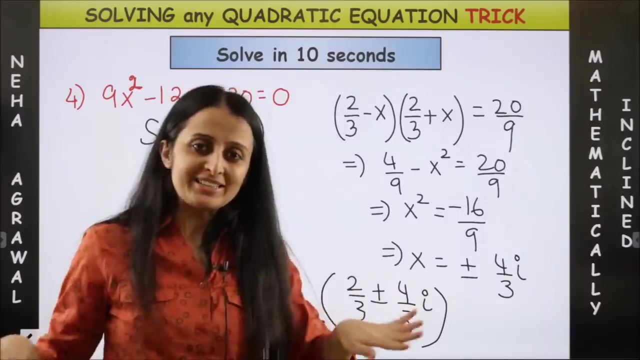 minus 16 by 9.. This is a problem. This is not a problem. This is the solution, Because x will be now plus minus 4 by 3 iota, Because square root of a negative number. Yes, So that means my factors are 2 by 3 plus minus 4 by 3 iota. Come on, let's finish the quadratic.